wake up, my beautiful artists. welcome back to my channel, art awakening. so in this video I'm going to go a little further into depth about finding value in color. I posted a video last year about finding value in color with Bill Murray, which some of you may have seen already. if you haven't, go ahead and. 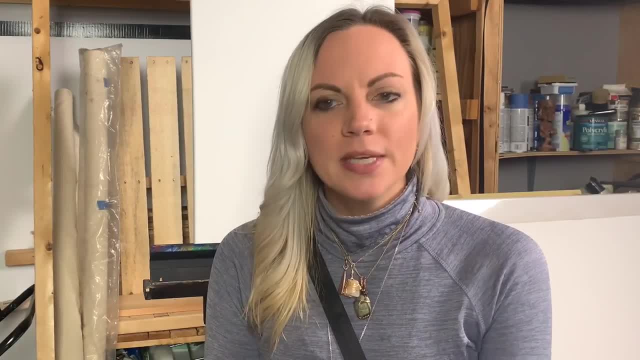 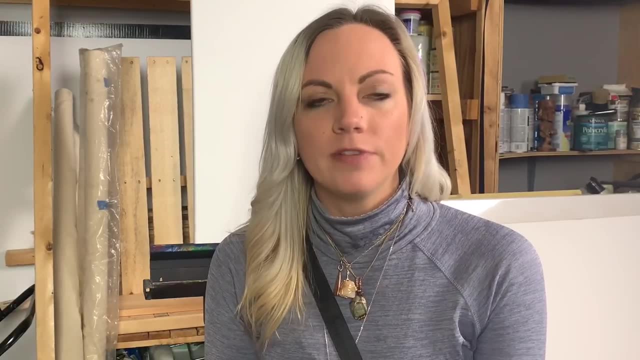 click that link so you can go check that one out first. this one's going to basically just be a test for us to kind of look more in depth into all of the different colors. I'm going to find the value in color of all of my Lucas paints. 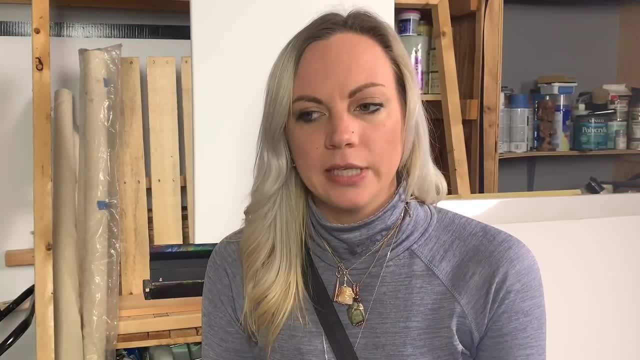 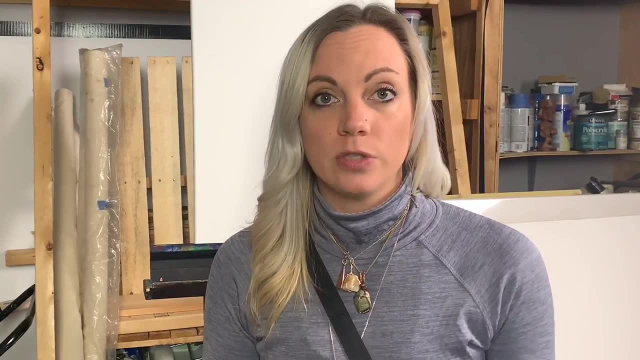 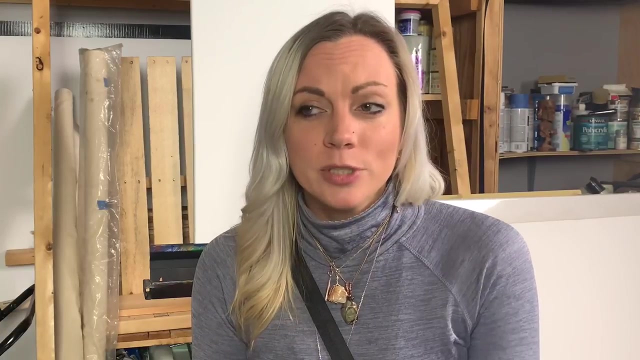 so in my colorful portraits I don't actually add white or black, you know, to change the value of the color. I actually just use the color straight out of the tube. and I love using the Lucas paints. they're super high quality. I'm not being paid for this, by the way. I'm just telling you that I. 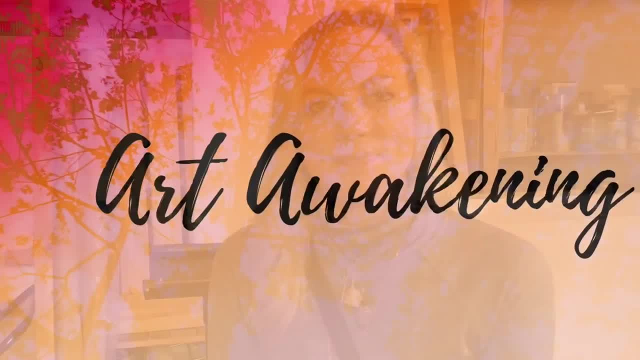 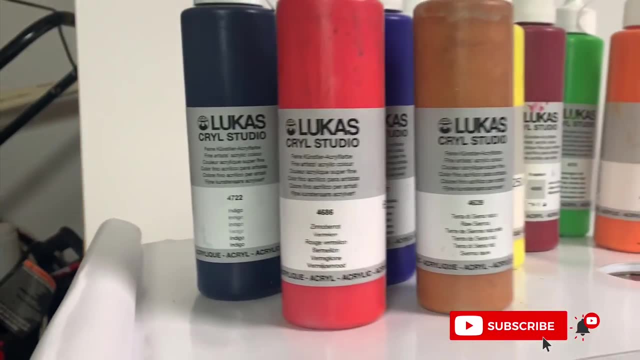 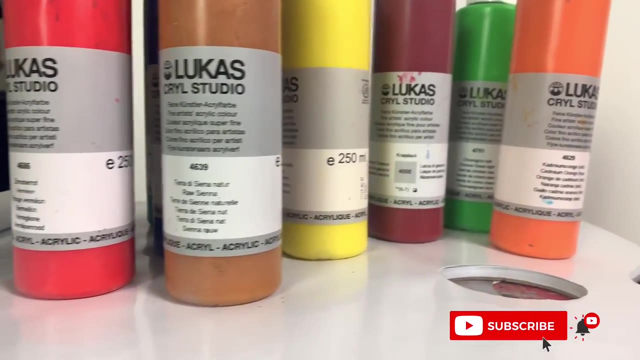 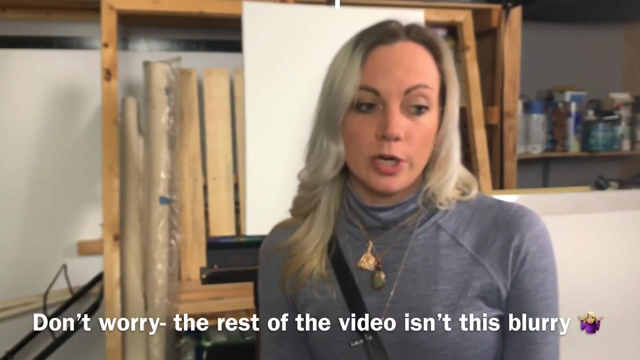 like to use the Lucas paints. I'm not being paid for this, by the way. I'm just telling you that I like these paints. so yeah, let's get started. so I'm going to use a couple things in order to make this process go a little bit smoother. I'm going to use this grayscale and value. 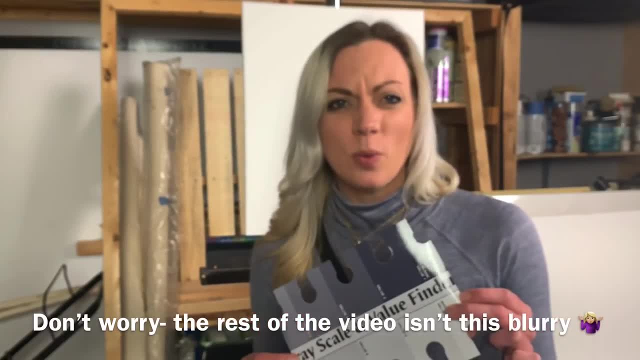 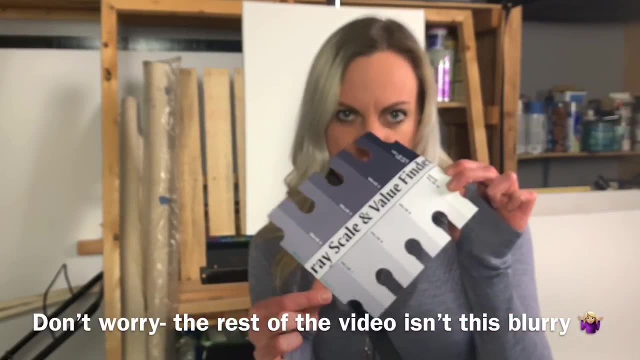 finder. I know it didn't print the whole thing. I tried to print it twice and it printed out incorrectly and I can't seem to figure that out. so this will work, though you can still see all the values. I just, you know, wrote in the little extra values here. I'll be fine, you'll understand, and I'm going to use my iPad. 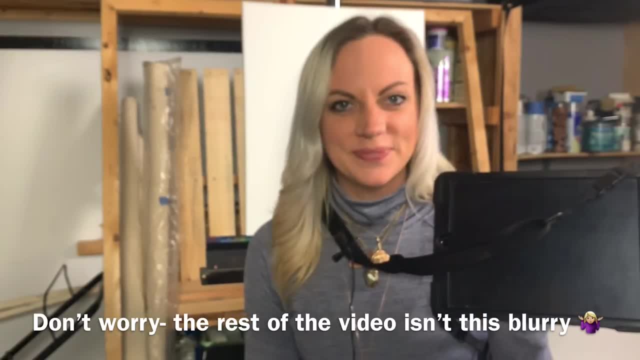 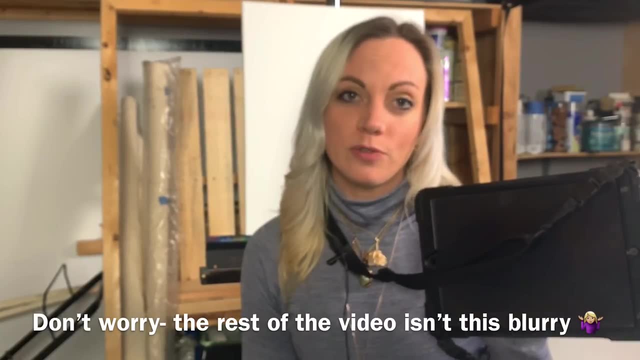 since my phone is recording me right now, I'm going to use my iPad to take photos of the colors and we're going to put those photos in black and white- kind of cheating. but at least it kind of looks nice, if it does look a little bit better. 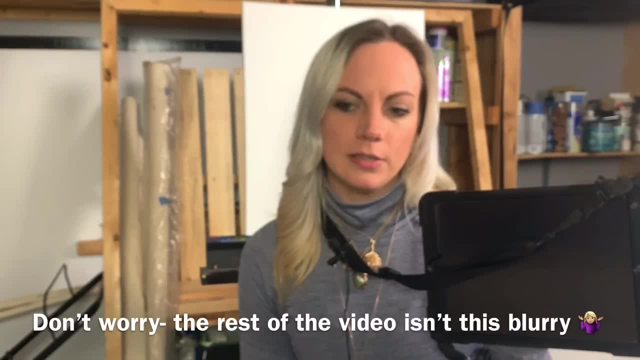 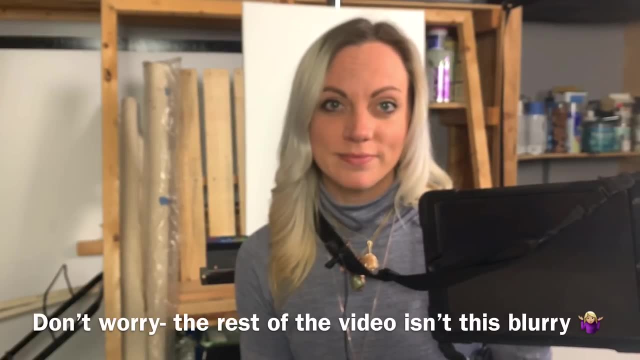 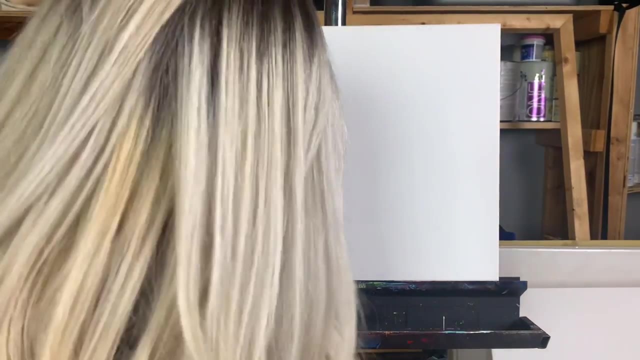 kind of gives you an idea about finding the value, and we can, you know, test to see if we can find the value. then put it in black and white and see if we got it correct. okay, so, while I get as some of this paint down on the canvas, here I did. 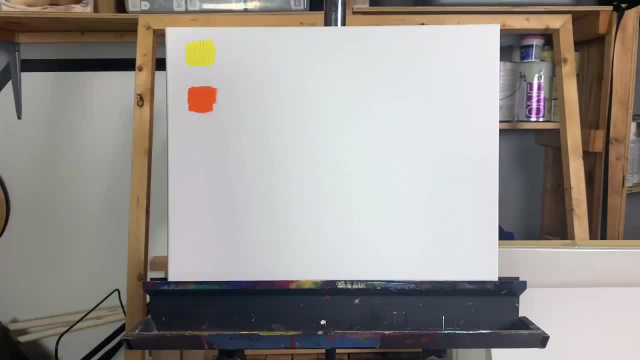 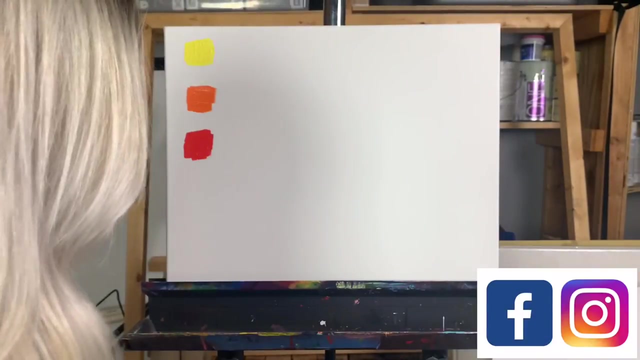 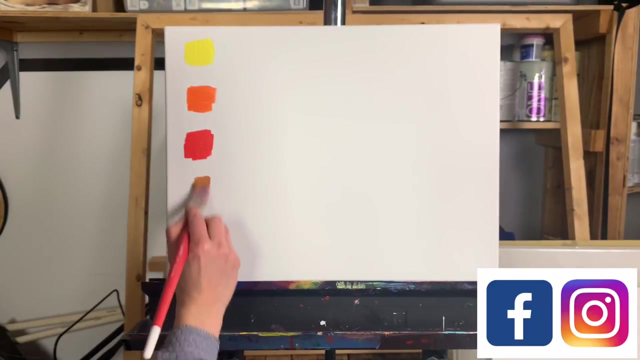 speed up this video so that it wouldn't take forever. I had to rinse my brush every single time that I change colors here anyway. so value? value is defined as the relative lightness or darkness of a color. it is very important for the artist in the way that it defines form and creates spatial illusions also. 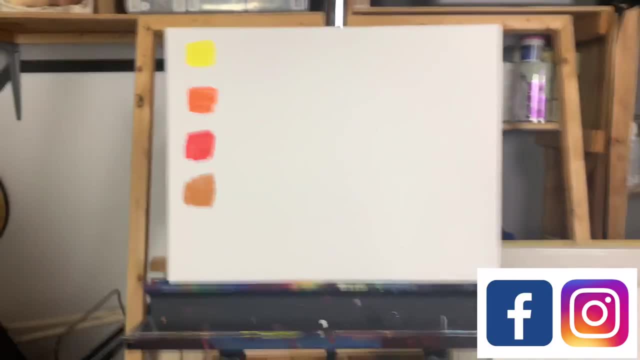 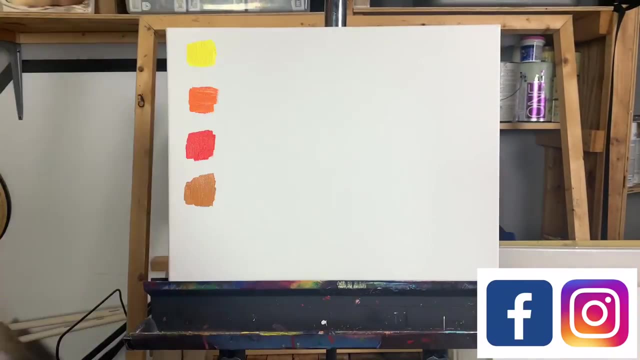 contrast of value separates objects in space as well. optical illusion type stuff. it gives you like light and depth. you can see that the color is a little bit different, so it's not necessarily. I don't know how I came up with this and my idea for it is to be a little more. 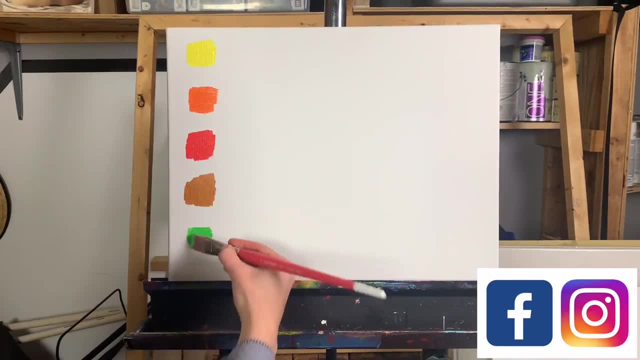 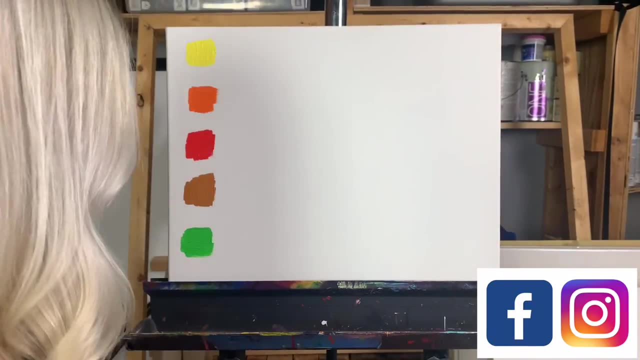 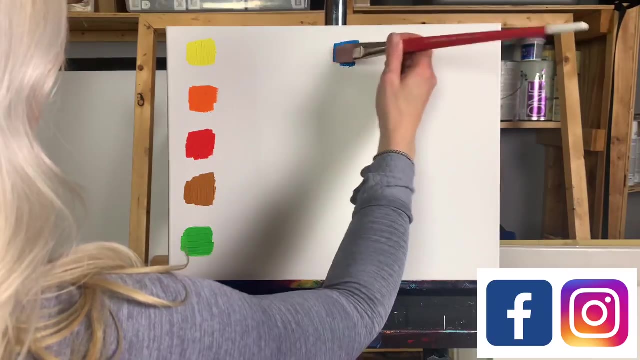 and form, So I'm going to keep putting this paint down. I'm actually going to skip through the rest of this and see in just a second. Actually, hold on Before I go. the bottom right-hand corner of Facebook and Instagram. be sure to follow me on Facebook and Instagram. 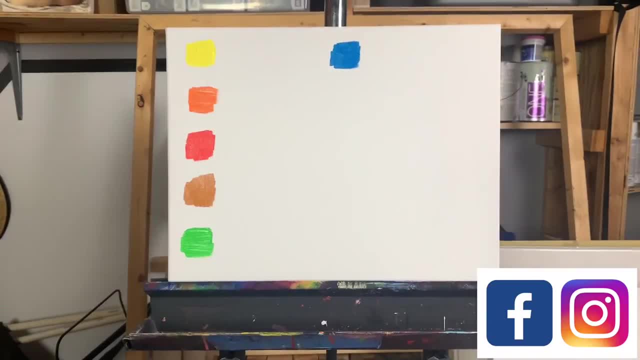 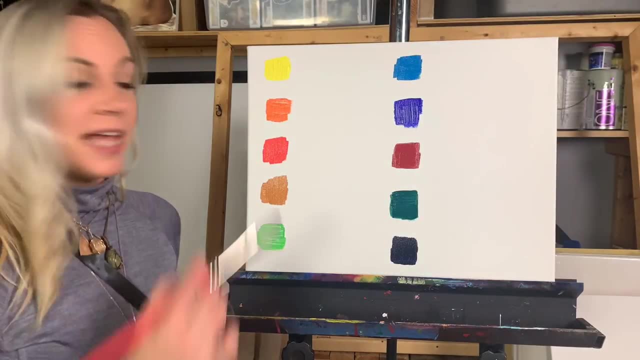 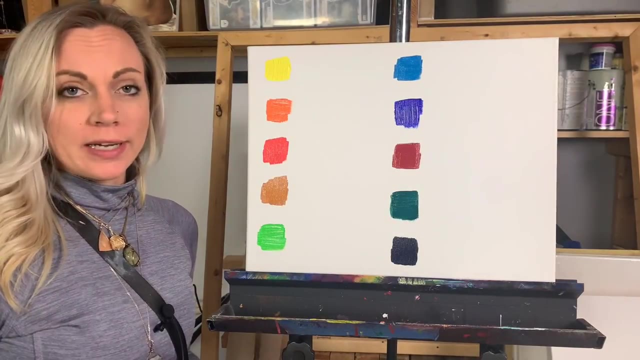 at Art Awakening. It is at Art Awakening for both of those platforms. Okay, So now I have all 10 of my Lucas colors down. I kind of put them in order, but not really. We're going to test that out right now. Actually, before I start on this with 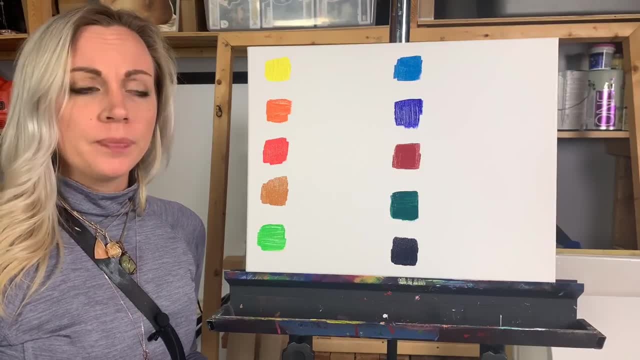 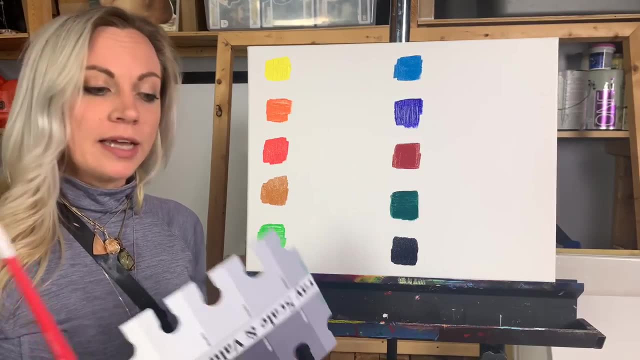 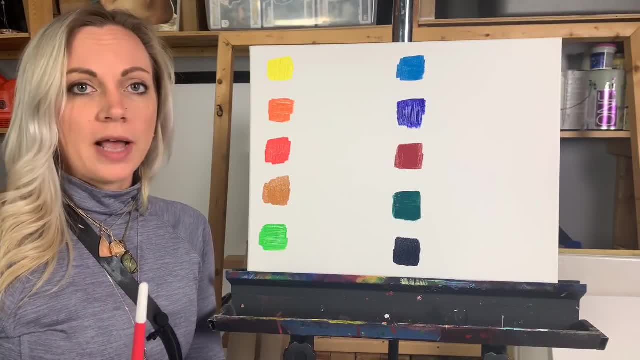 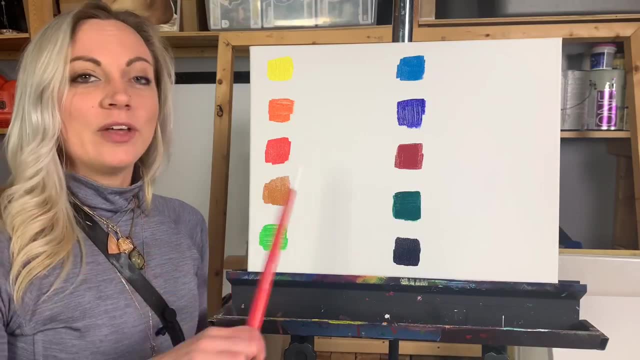 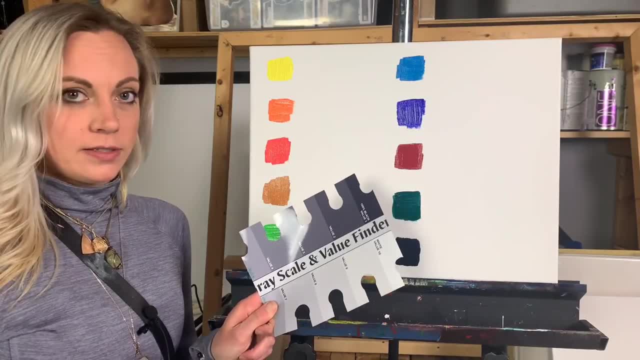 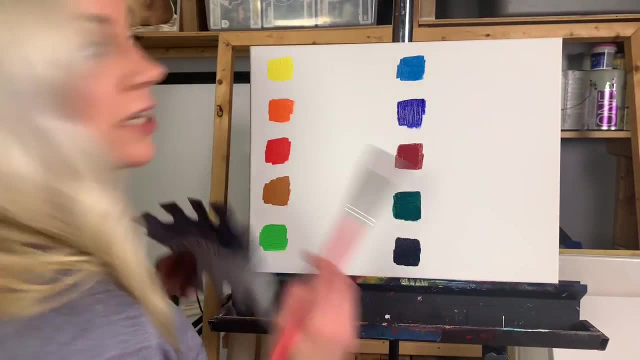 what I was saying. Here's my silly value finder that's halfway cut off on both sides. You can still have the colors, still the values. Don't do that, Anyway. so we're going to start with the yellow. So I know that it's one of these lighter colors. 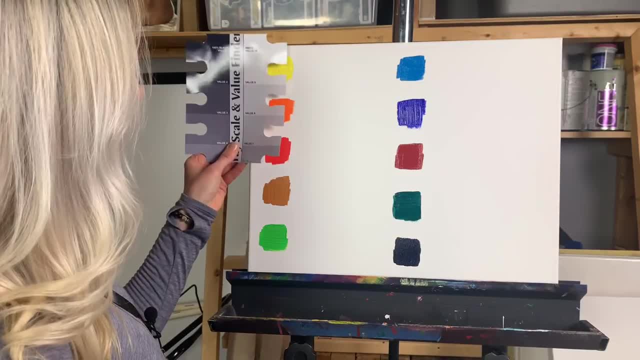 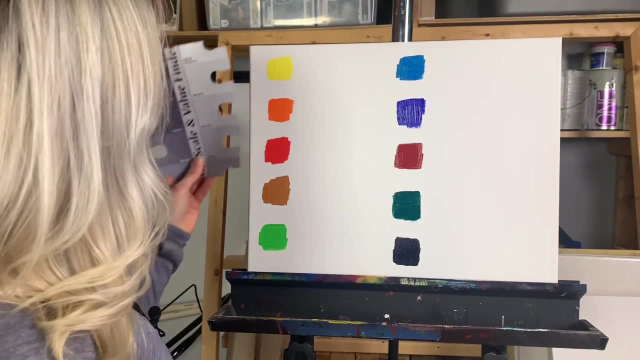 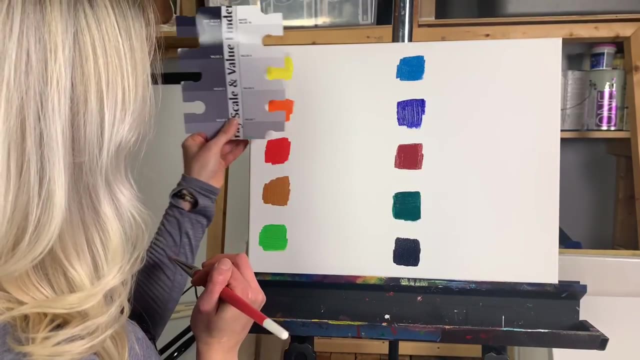 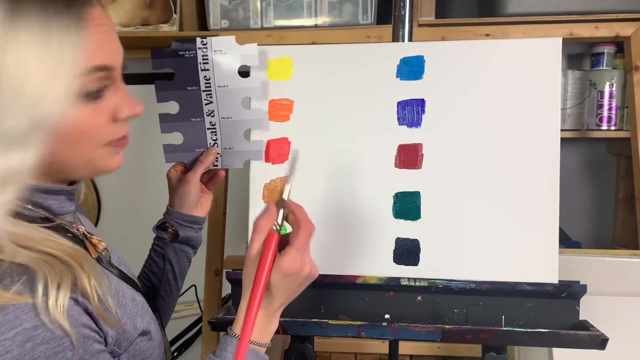 I'd like to say it's probably a value nine. So we're going to go with value nine for that And I'd say the orange- if you look closely the orange kind of matches this value here. It's a little bit too light to be in the value seven. I love these little notches here. It. 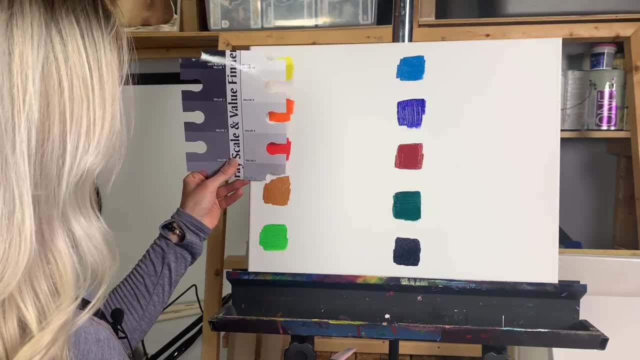 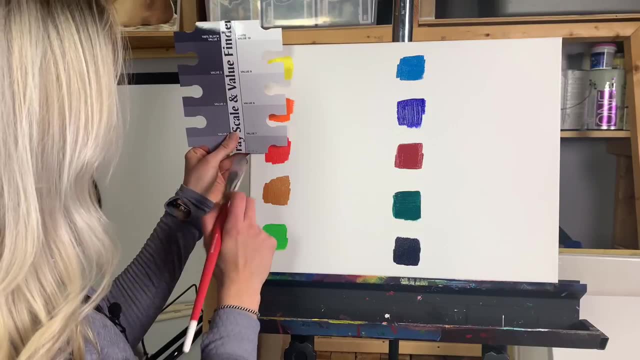 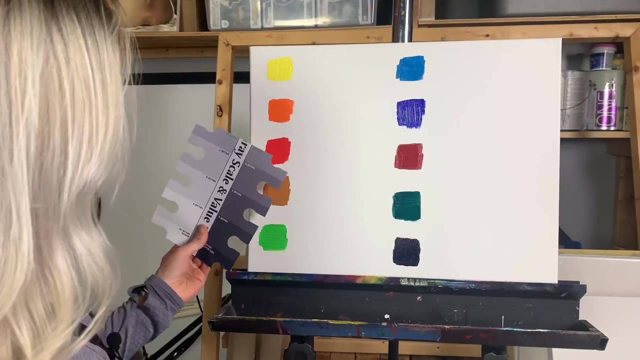 looks like it's going to be a little bit too dark, So I'm going to go with a little bit of orange And I believe we'll be. could be a value six. Actually, this value right here, I could say that it would probably be close to a value six. All right, Let's see. I'm thinking that the brown 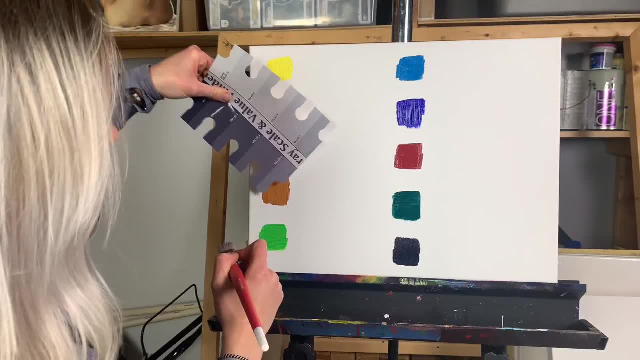 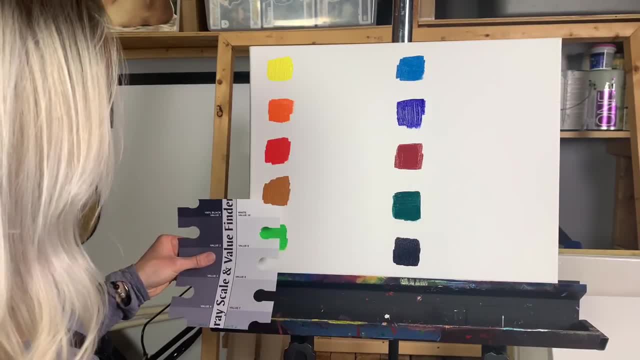 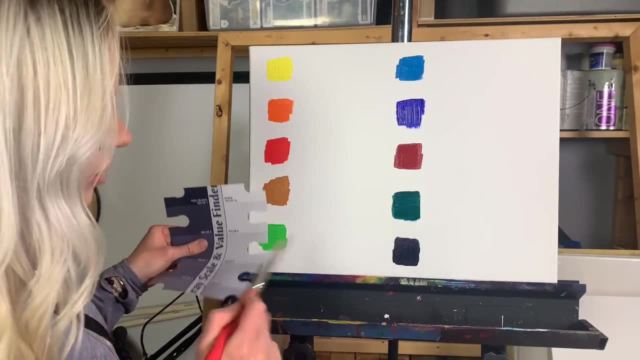 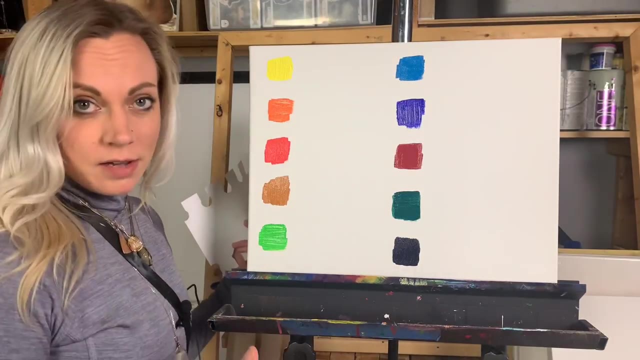 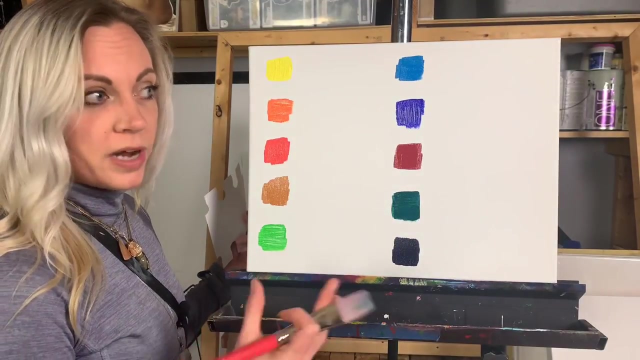 looking at again, And the green, I mean it's a very bright color. So what you need to do is you need to kind of understand that the intensity of the color, the brightness of the color, in finding value does not matter. So you need to kind of train your eye to kind of overlook. 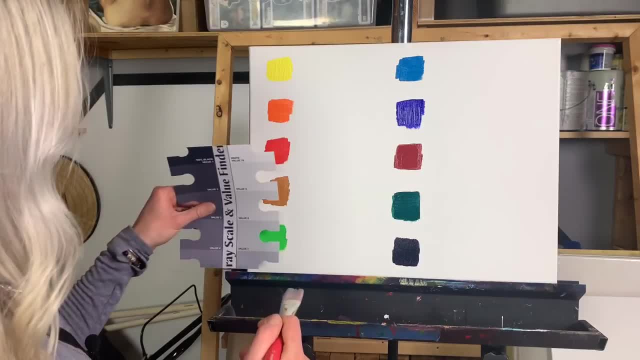 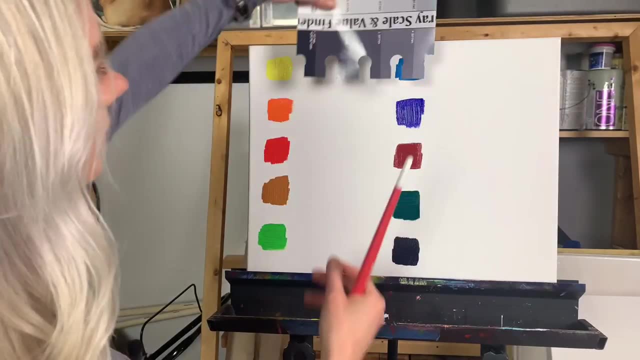 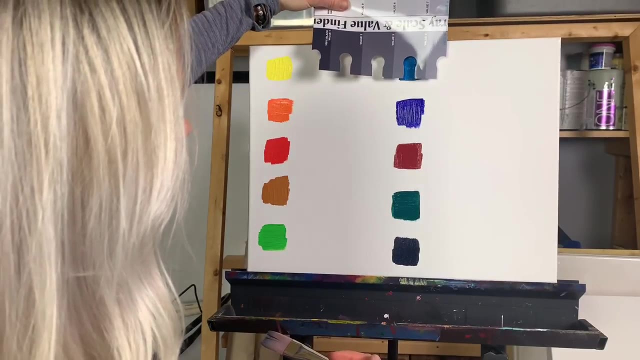 that part of the color, So the green. I'd say the green may be like a value seven, So let's go with seven. It's a bright color, the dark blue or the light blue, but you know it's not super. 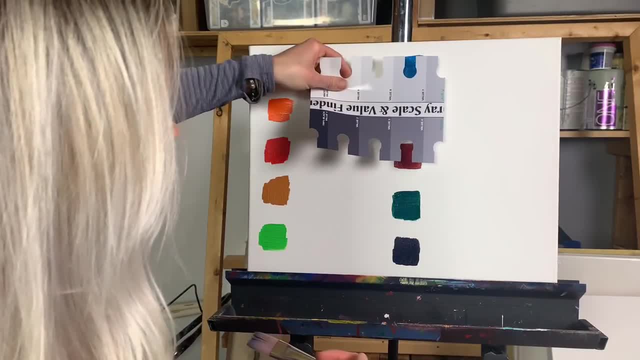 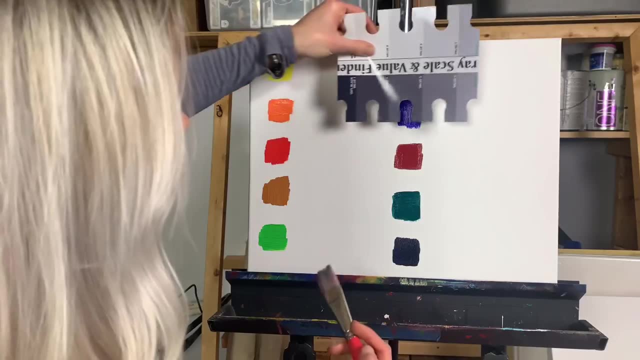 bright Like it's way too dark for that, Too dark for that, I don't know. Value four or value three? I'm going to go with the value three, All right, And we're going to go to this darker one here. Okay, That's absolute black, It's not? 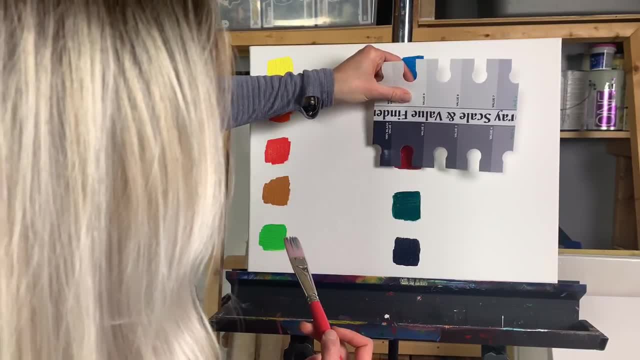 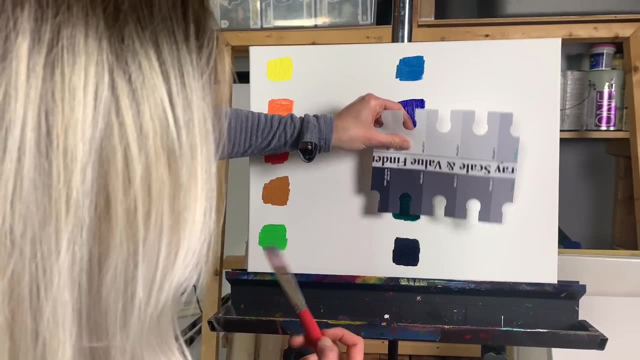 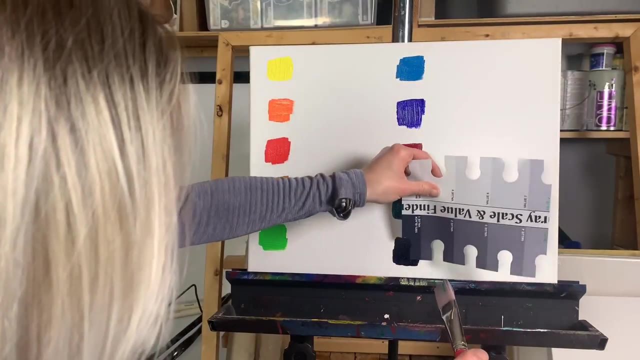 that I'd say probably value two for that. Probably another value two for the red and the green. I don't know. Let's see, I think of all these colors. I guess it's hard to tell. The green might be darker And value one, I say this one's closest to black for me, So all right, Let's put. 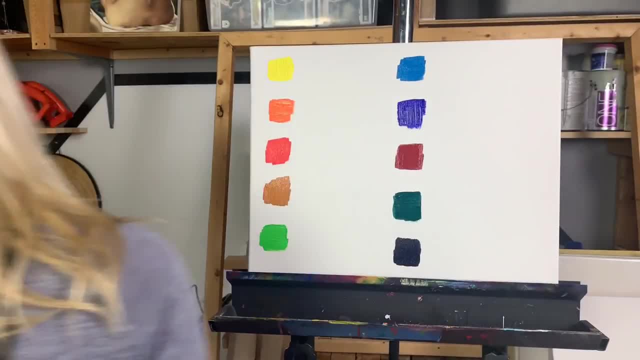 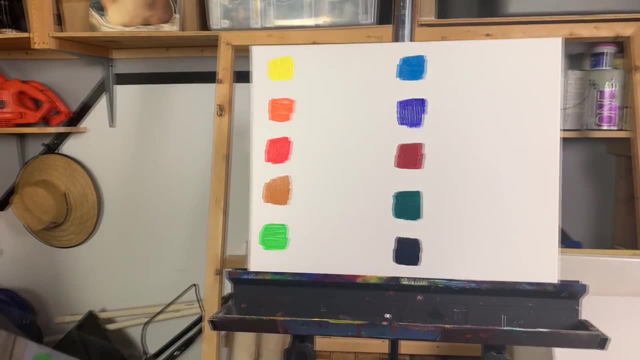 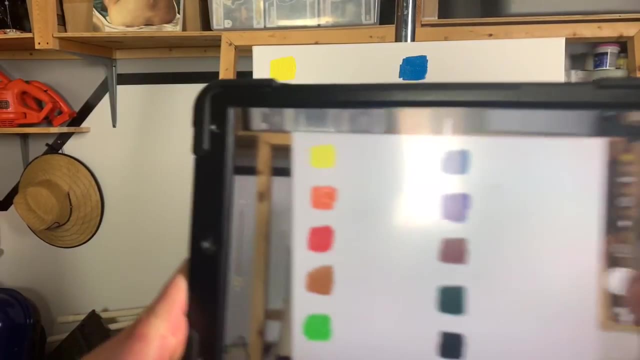 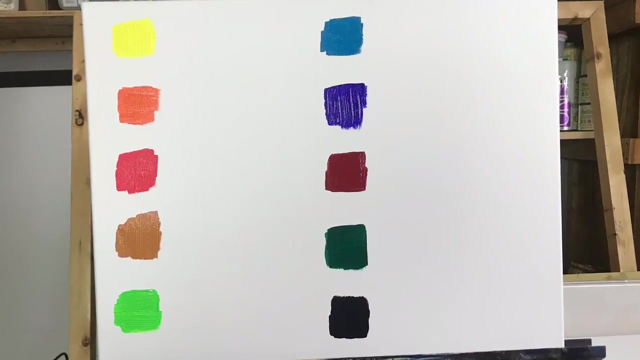 this in black and white. I'm going to take a photo of this with my iPad. that was attached to me and I totally didn't even realize. Okay, So I'm going to go ahead and take a photo which I will show you right now. All right, So here's our photo of all of my Lucas colors there. So I went ahead. 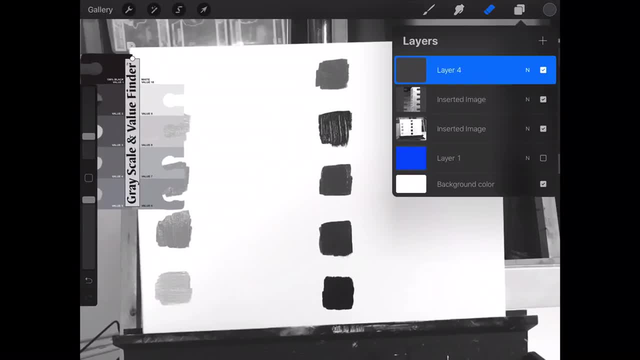 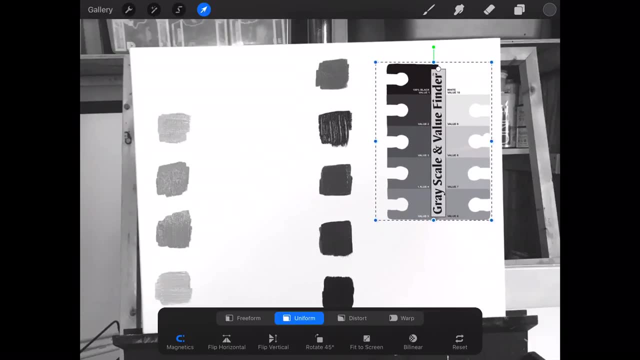 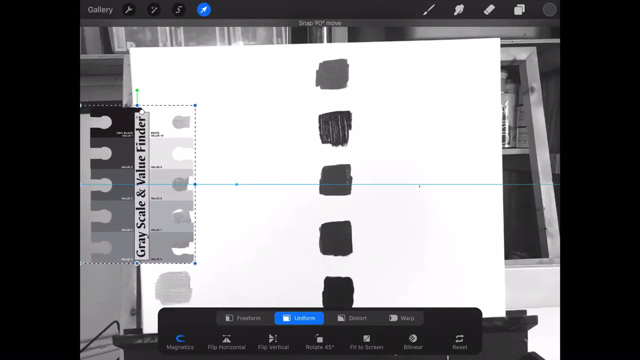 and put that in black and white, otherwise known as mono short for monochromatic- Just darks and lights there. So I also put my little grayscale and value finder in here digitally. I thought that this would be an easier way to show you, So we're going to see how this goes. I also had to adjust. 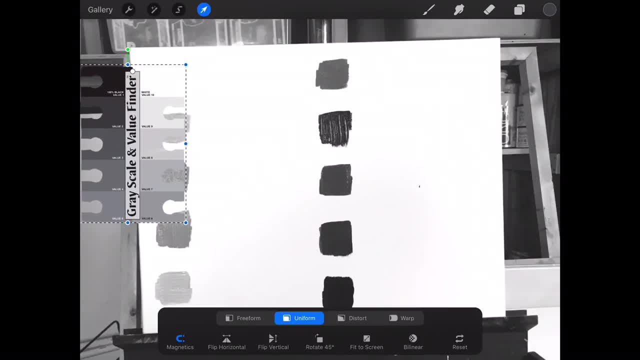 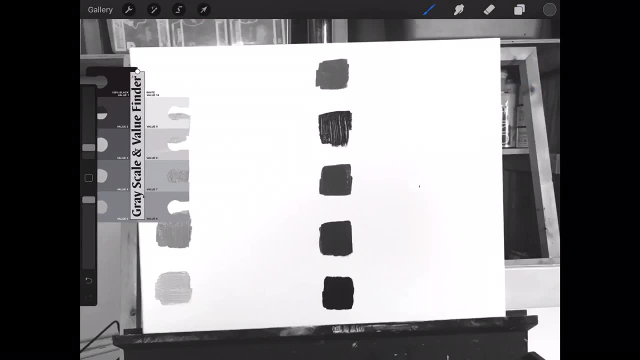 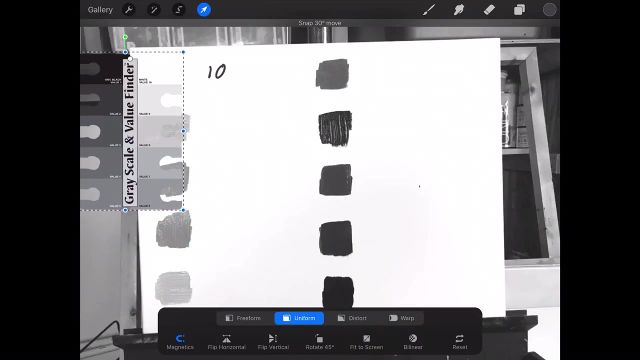 the white balance of the photo to get it to be the particular white color that I was looking for. And, as you see here, the first color here the yellow with the first value. So that is definitely definitely a value 10.. So the second color here. 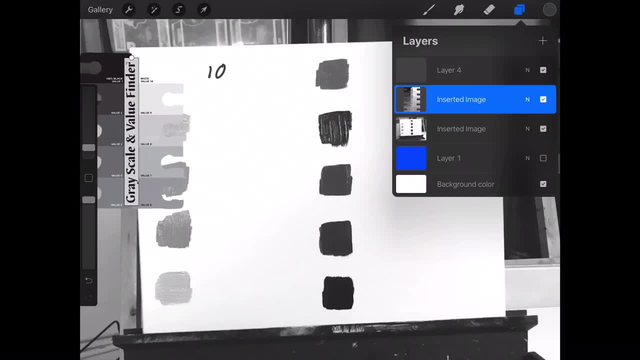 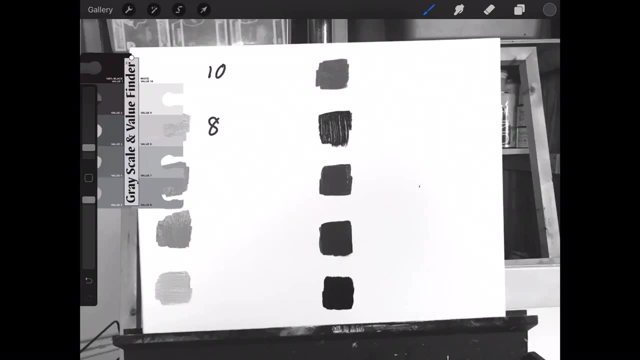 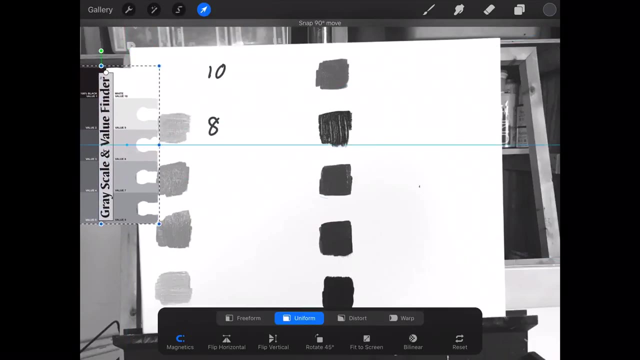 and we're going to go through and remind ourselves which colors were, which I believe this was orange. This one is actually a value eight, not a value nine. You would think it might be a value nine, but it's actually a value eight. I sped this video up just a little bit, you know to make. 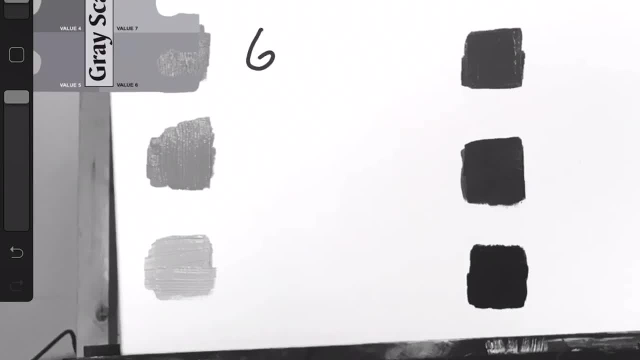 this a little bit easier for us, All right. so I just went ahead and zoomed in here for you so you could see this a little bit better. That one is definitely a value six. It definitely matches. I had it in the wrong layer. 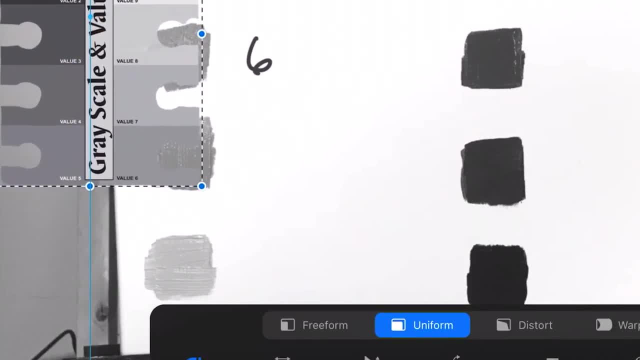 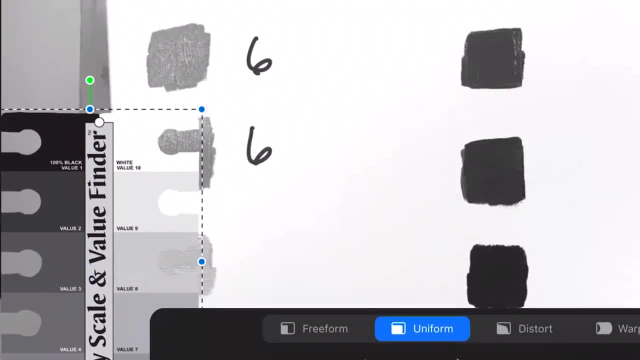 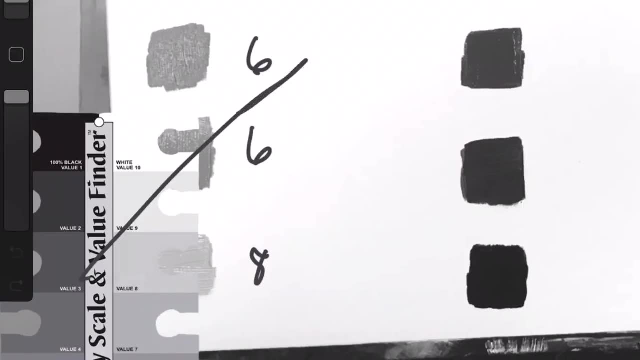 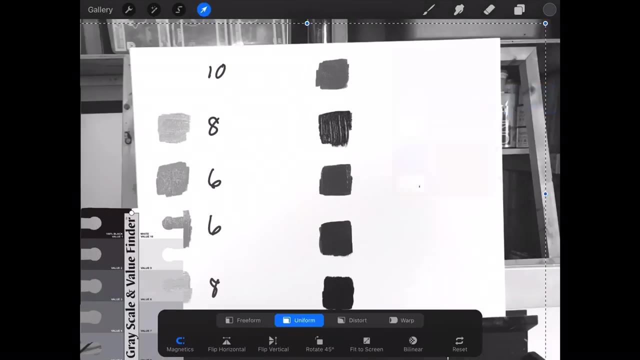 that I came up with earlier in the video And we're gonna see how well we did. It's kind of like a test to see how we did. I don't usually use the numbers like this when I paint, but I might actually look into doing this more often. 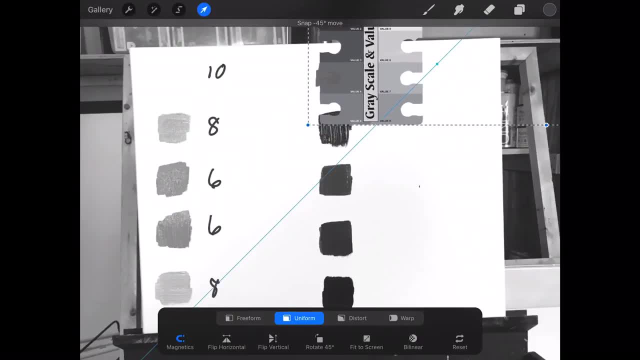 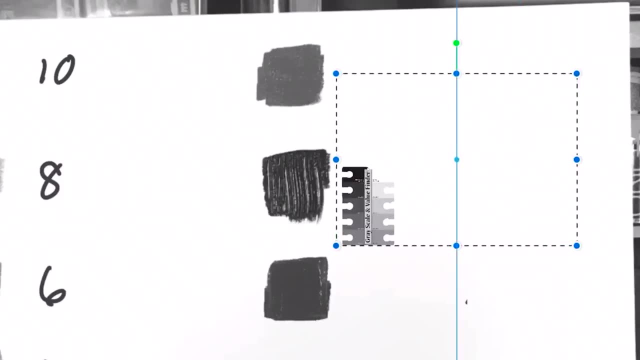 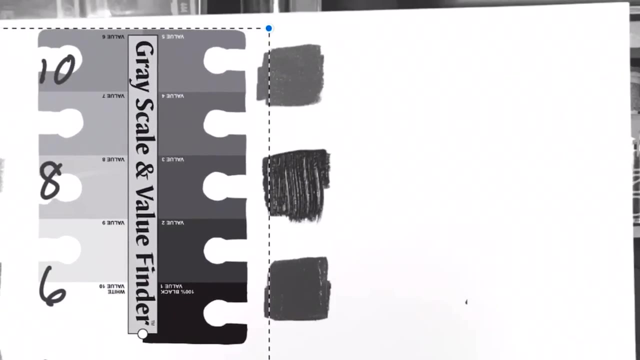 It's very helpful, So let me zoom in for you one more time. Okay, so this one here is gonna be a value four. I'm gonna go ahead and turn this around. You know I had to digitally cut this out in order to use it this way. 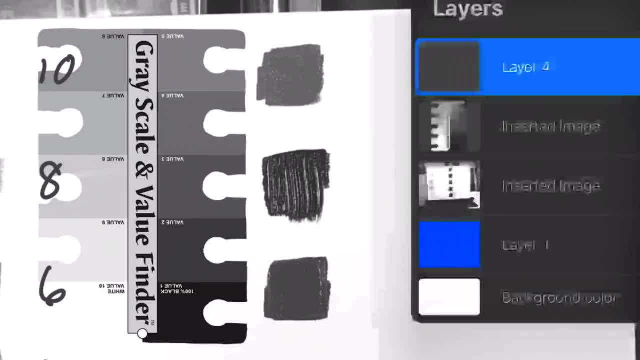 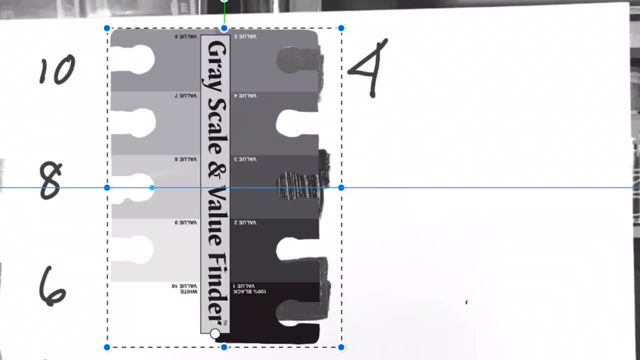 Thankfully, it didn't take me that long, which is pretty good. I love Procreate. This is what I'm using, the platform that I'm using right now, or the app that I'm using right now, rather So the next one. you see how it has. 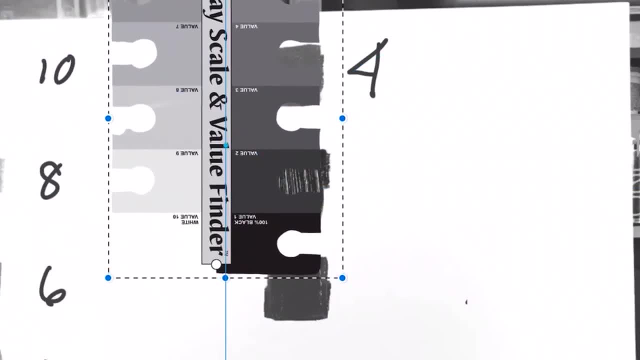 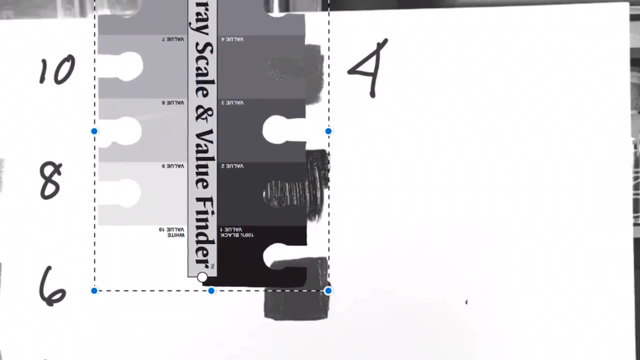 the kind of the light spots in there. That is actually the reflection of the light, since it was fresh paint on the canvas. So we're gonna go ahead and ignore that And we're gonna take the darker part of that color, which is definitely going to be a value two. 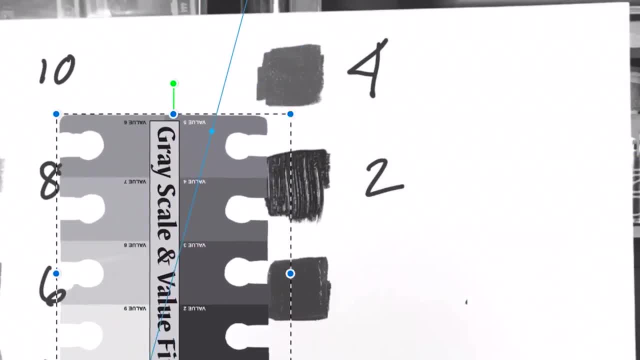 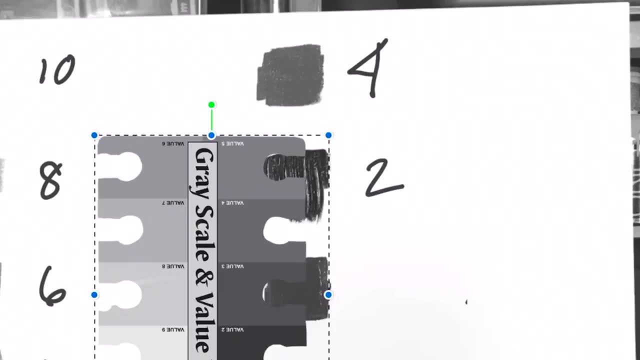 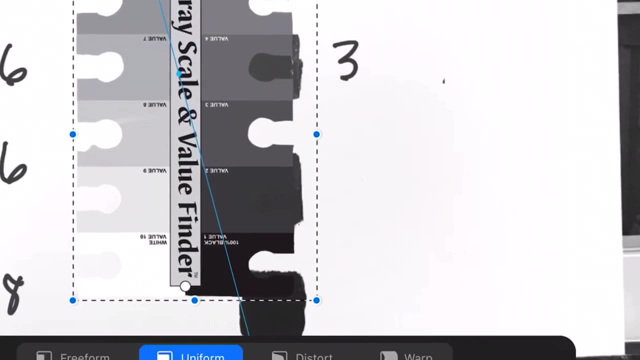 So we're gonna go ahead and write two there And Third one down here. That is definitely a value three. See how that matches up super well. So we're gonna write three Right now for the last couple of colors here. Oh, 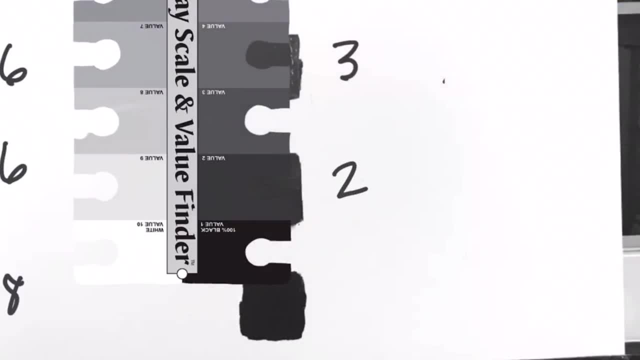 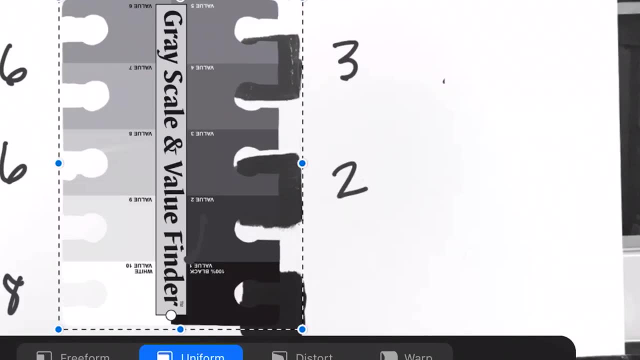 perfect, value two, absolutely. and then the final one there at the bottom, the dark blue, which is what it technically is, and that's closest to a value one, maybe between a value one and a value two, but we're just gonna go ahead and put one there for now. 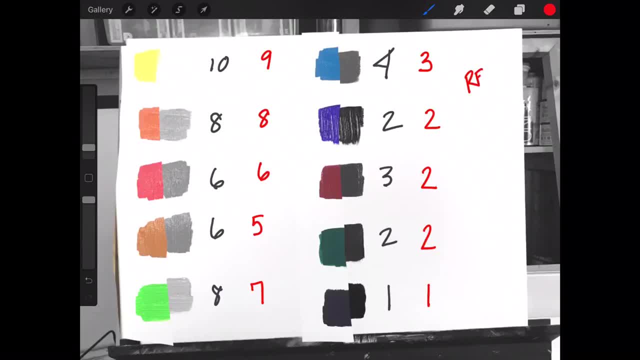 all right. so here we are, and I actually went ahead and I took the colors from the original piece and put them right next to the values so you can actually see this together. I love how I can do this digitally and actually see them side-by-side without any hassle, so you can see, kind of, where we went right and